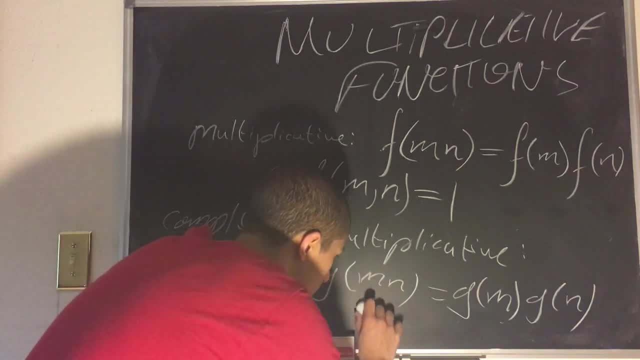 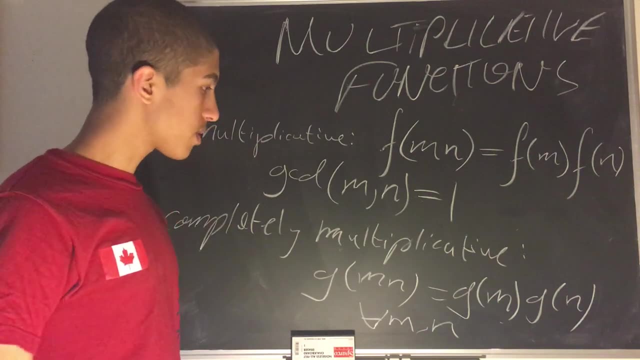 which is not met in multiplicativity. So for for all m and n, for every m and n, that is, And physically we're saying that gcd testi can be multiplied by perfect comma n, And so we can see right away that simple multiplicativity is a much harsher. 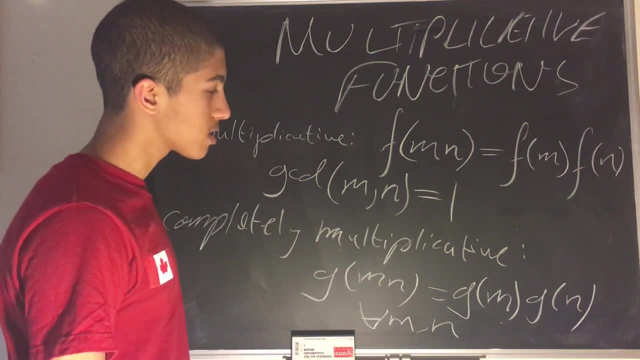 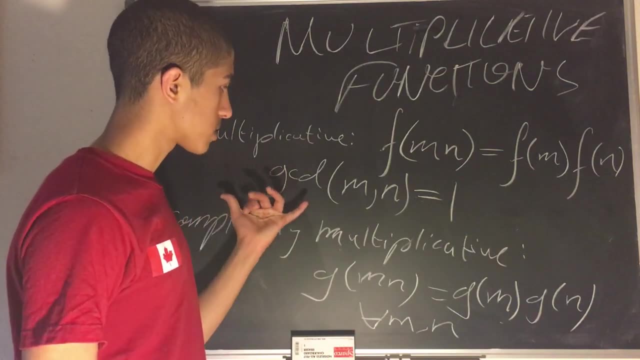 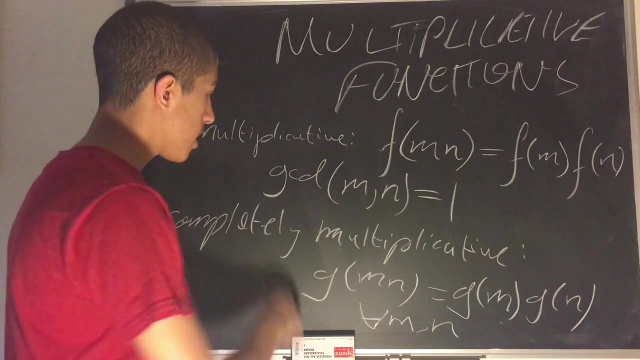 restriction than complete multiplicativity. Actually, no, no, no, excuse me- Complete multiplicativity is much more open, whereas simple multiplicativity is much more restricted, because it necessitates that m and n are both relatively prime. And if you're confused as to 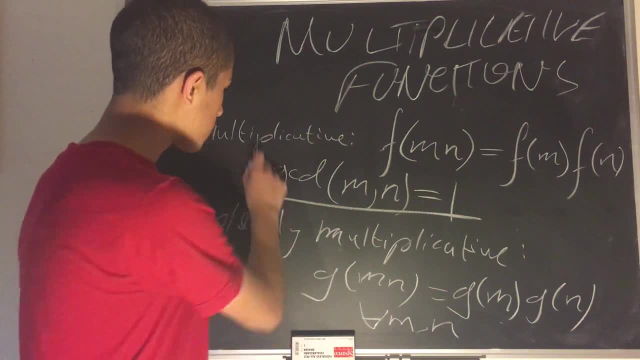 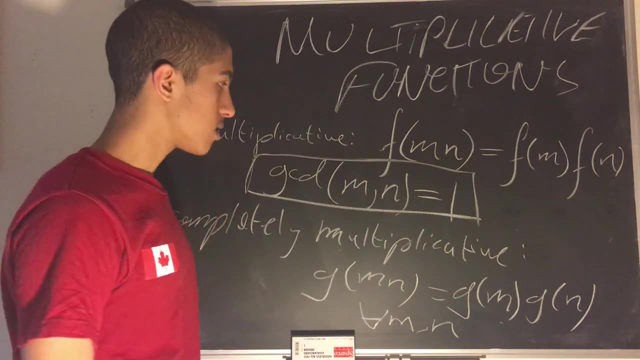 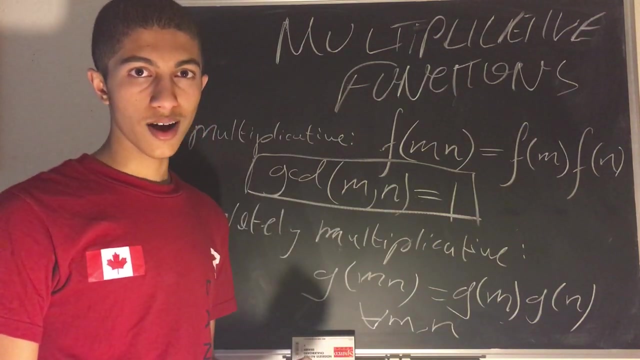 why I am calling them relatively prime. it's because of this, It's because gcd of mn equals one. Well, what does that mean? That means that the greatest common denominator, the one factor, that the greatest factor that both m and n share in common, is one. It's nothing else. So, for example, 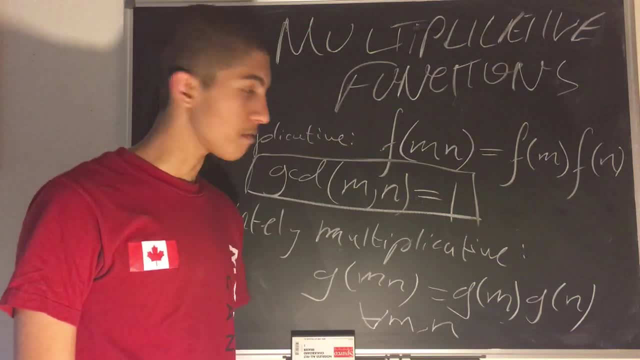 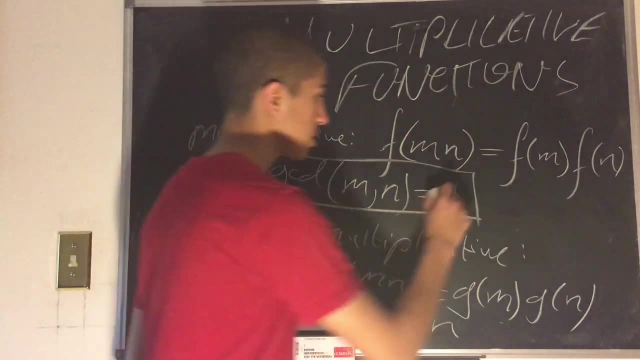 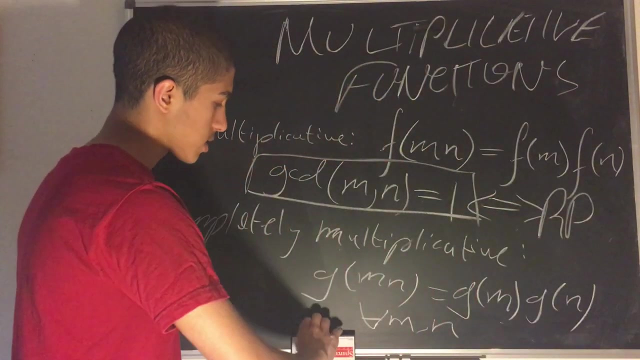 six and five. They're relatively prime because they don't share any factors in common other than one. So when you don't share any factors in common other than one, you are relatively prime. So this statement is equivalent to relatively prime, or sometimes called co-prime. So that is the 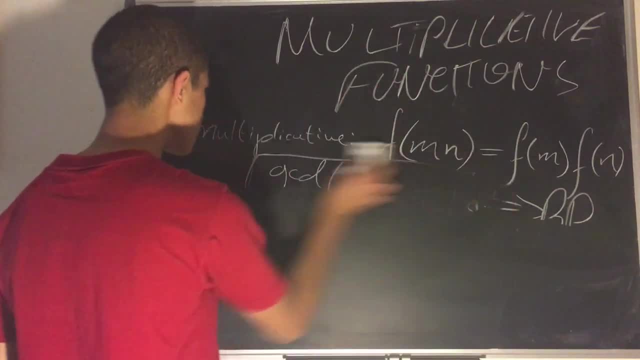 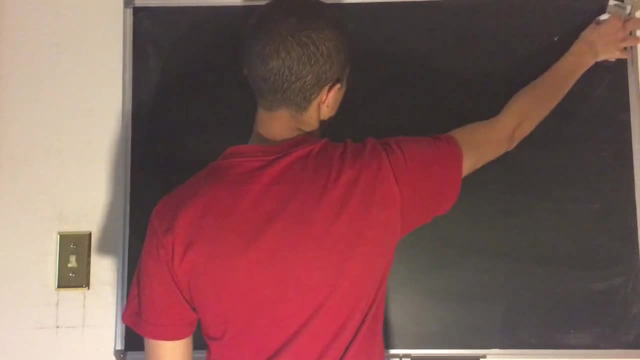 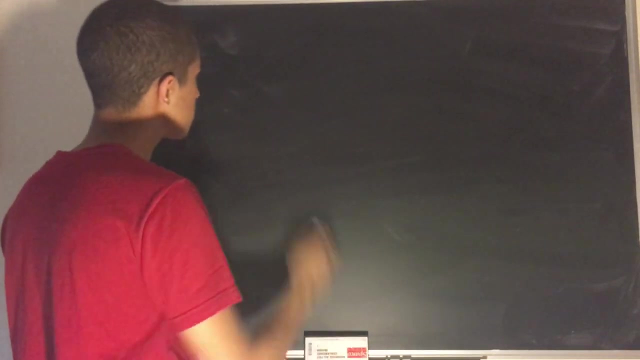 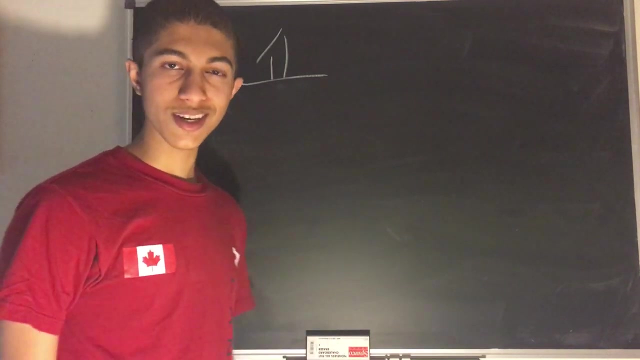 definition of multiplicative and completely multiplicative functions. So now let's discuss: well, what are some examples of some multiplicative or completely multiplicative functions? So let's let's ask ourselves. Let's discuss the function boldface1, which I discussed previously in my previous videos. 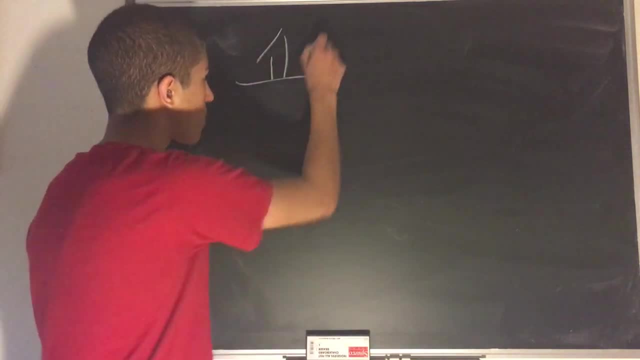 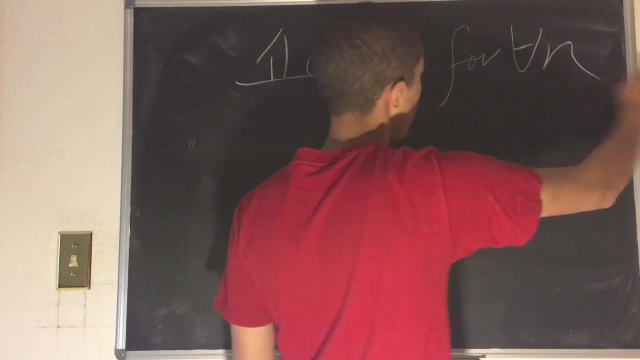 as my favorite function, and it still is, because it's so simple. It's wonderful. One of n is equal to one for all n. What a wonderful function. So let's ask ourselves: how will you be able to solve this? How would you do it this time? 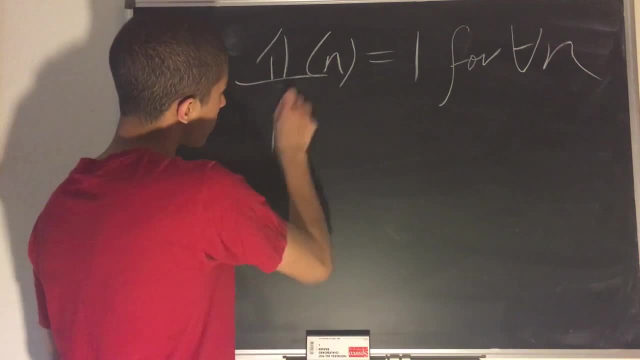 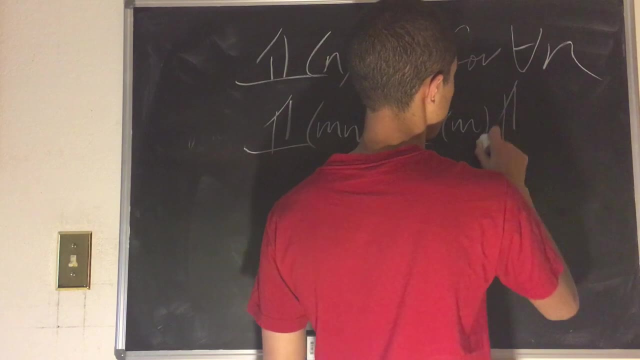 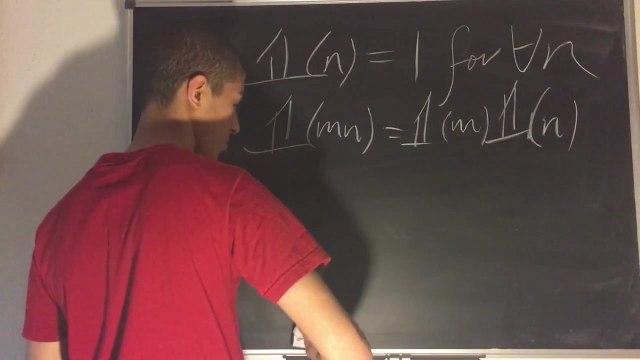 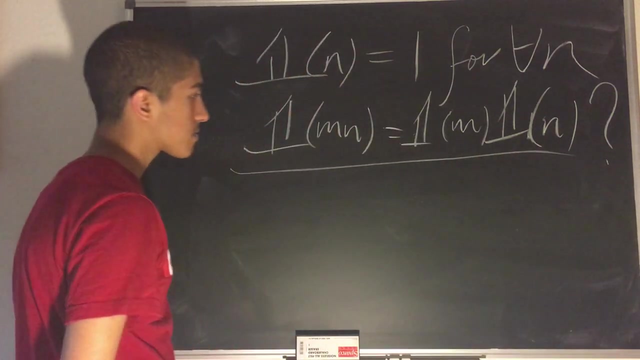 ask ourselves: is this multiplicative? and when we're asking that, it's equivalent to asking: is one of m n equal to one of m times one of n? that was a very bad question mark. let me rewrite that question mark much better. so, uh well, let's ask yourself: is this condition satisfied? is this? 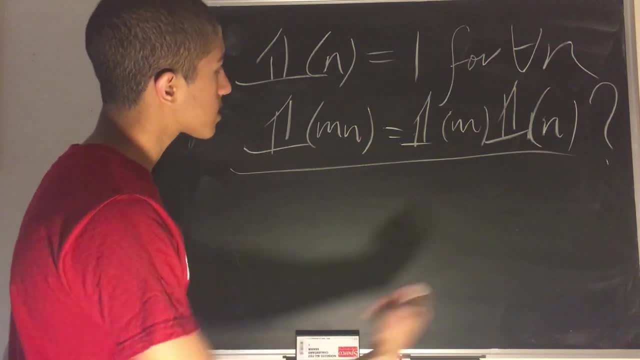 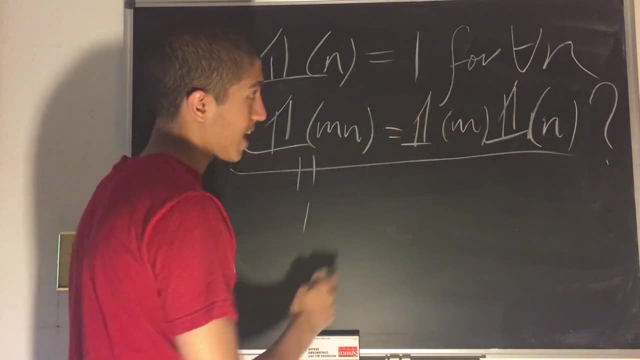 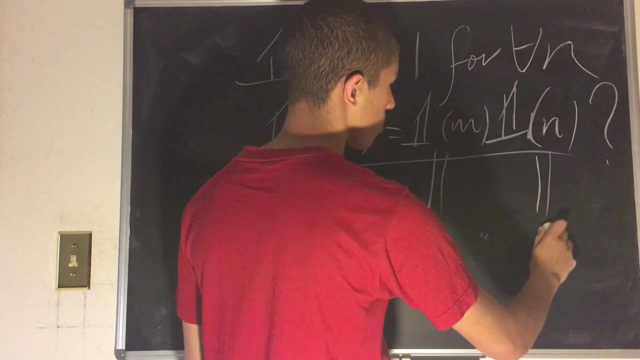 condition met? and yes, it most certainly is. and let's ask ourselves why. well, one of m? n is simply equal to one, because m? n is a normal number. uh, well, it's a number and, uh, it is equal to one. and one of m is equal to one and one of n is equal to one, so one is equal to one times one is this. 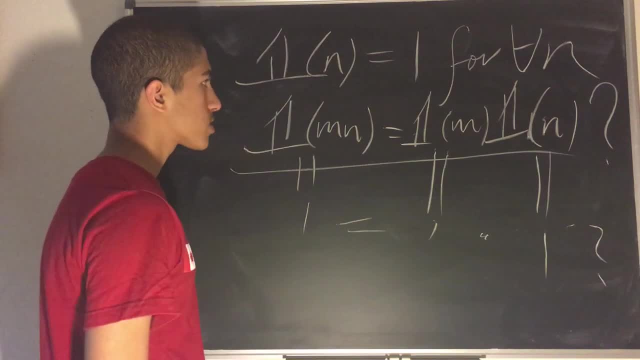 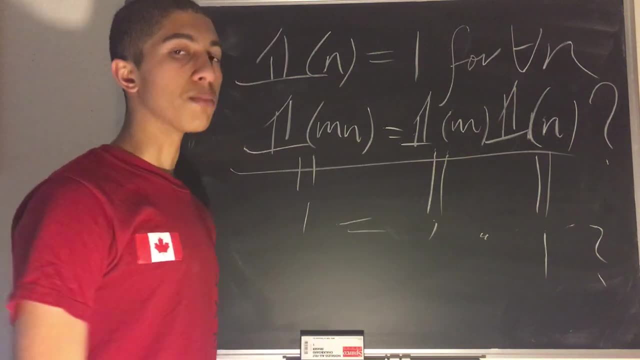 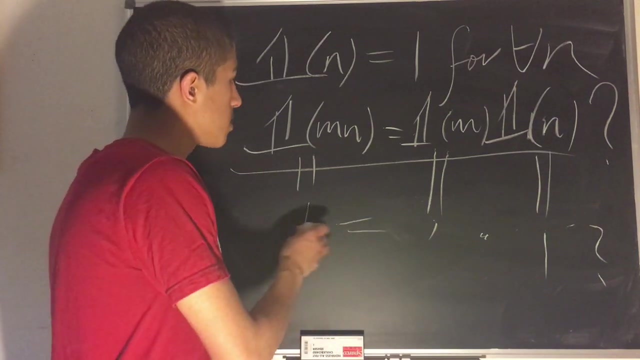 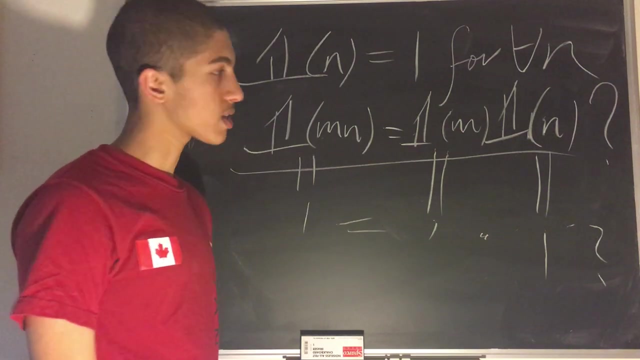 condition met? most certainly it is. so we can conclude that, uh, one of n, the, the function bold face one, is most definitely multiplicative. But the question is: is it completely multiplicative? Well, yes, of course, because m and n if they're not co-prime, if they're, for example, if m equals. 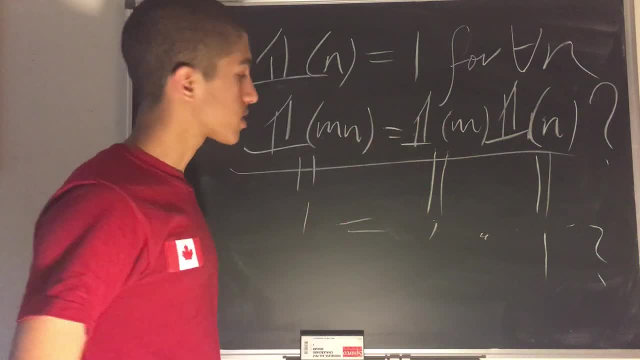 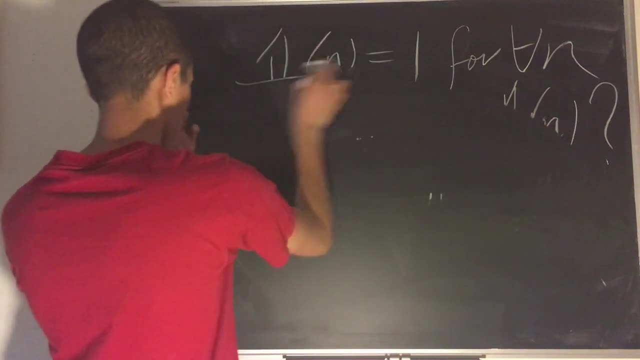 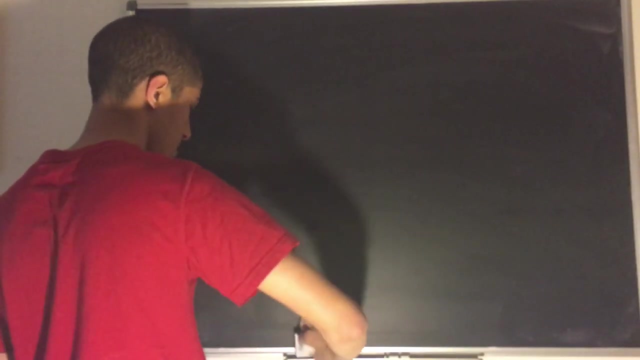 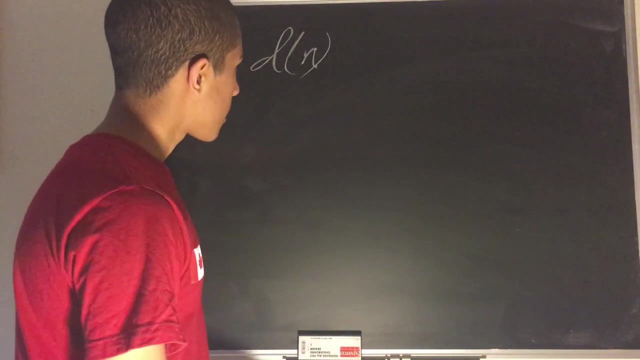 n. this still holds. This holds for any m and n. So it is both multiplicative and completely multiplicative. And now let's ask ourselves: well, what about the function d of n? Is this multiplicative? Well, I will prove to you in a few minutes that it most definitely is. 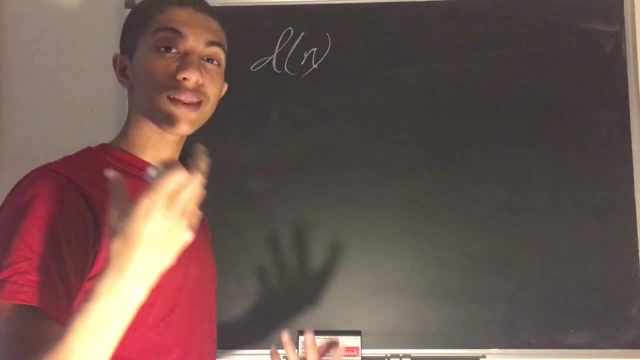 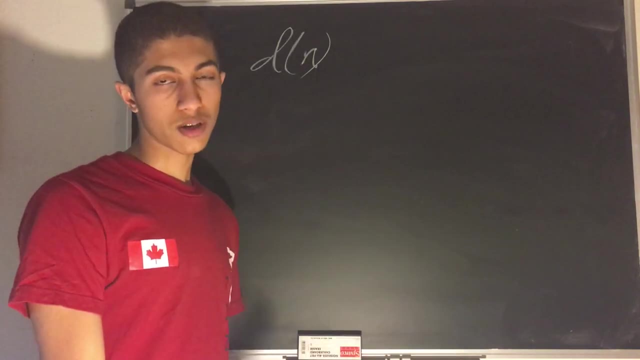 but there is a more general way to prove to you that a more general class of functions have multiplicative properties, whereas I could just prove d of n is multiplicative and each other function in the class is multiplicative. So let me show you right now. 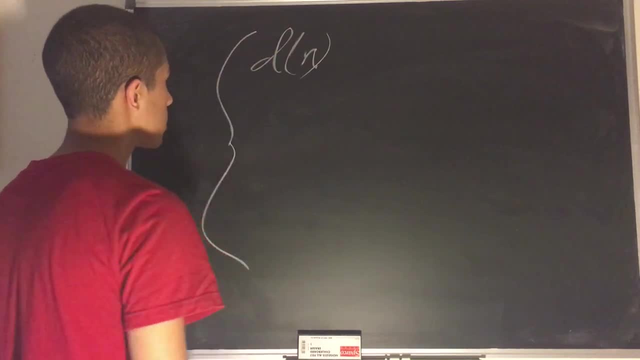 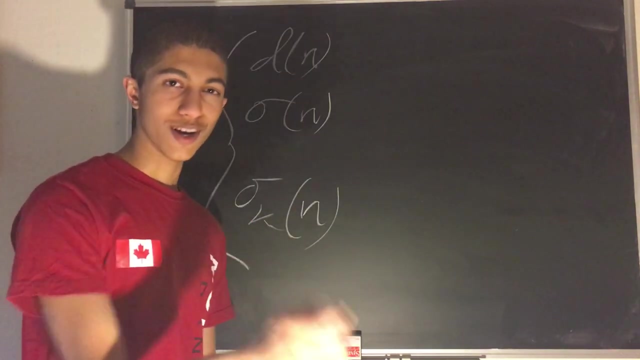 The questions we will be asking are such: is d of n multiplicative, Is sigma of n multiplicative And is sigma k of n multiplicative? And well, if you are very, very smart and if you are a bright young boy, unlike myself, 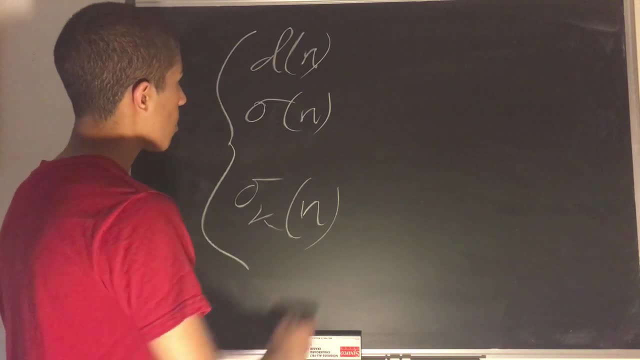 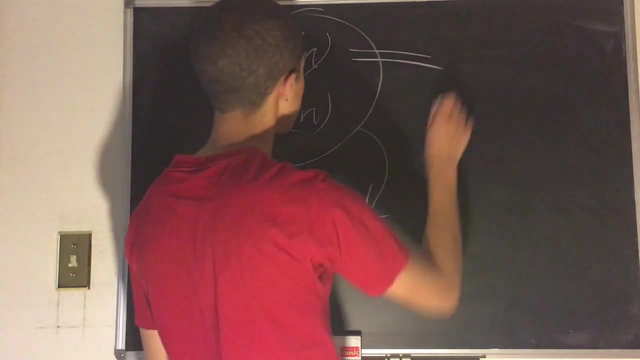 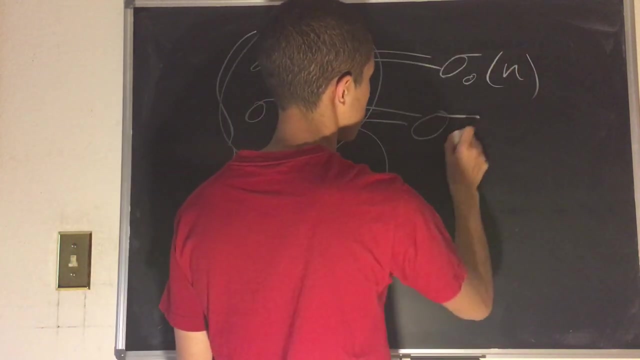 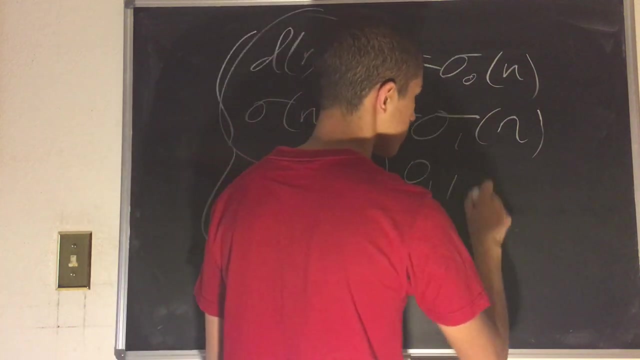 then you will definitely notice that both of these functions fall under sigma sub k, Because, if you realize it, d of n is simply equal to sigma sub zero of n And sigma n is simply equal to sigma sub one of n, And zero and one are definitely valid k's. 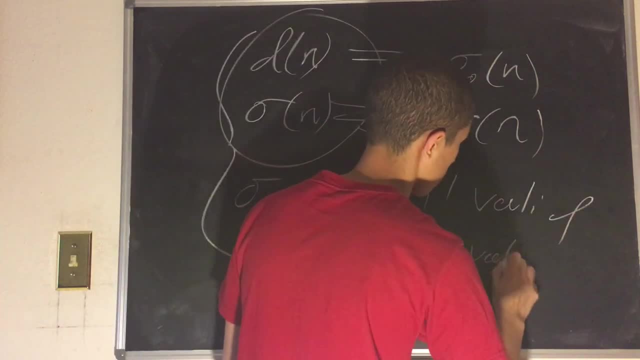 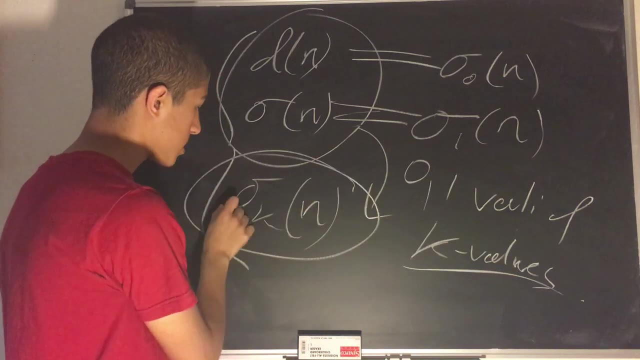 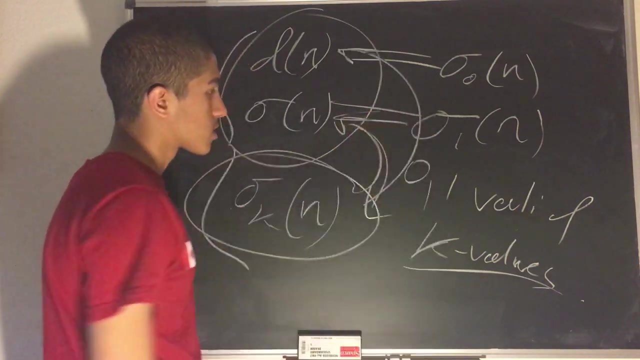 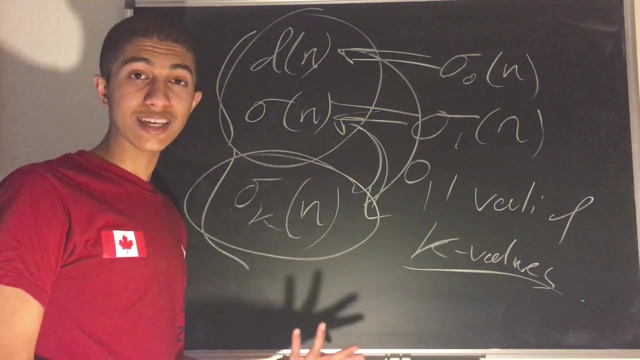 So we can most definitely just check that sigma k of n is multiplicative, And that will imply that both of these two are multiplicative. So that is why you would not want to prove each of these separately, that you would just want to prove the last case and say that it applies for both of the 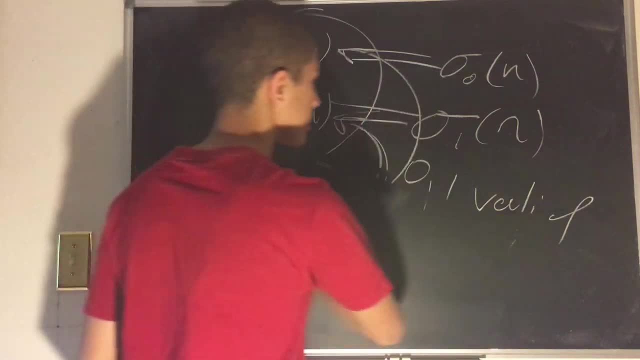 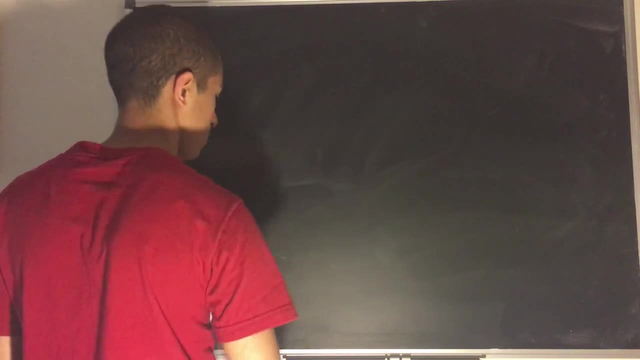 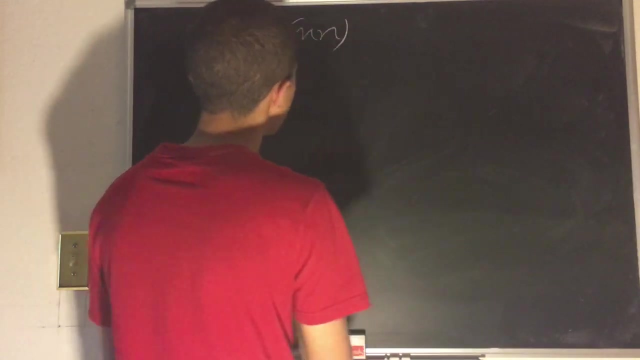 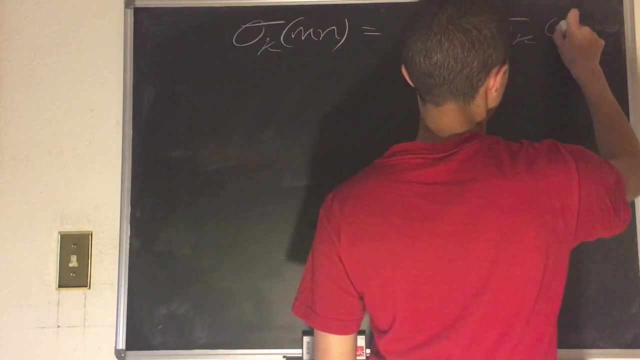 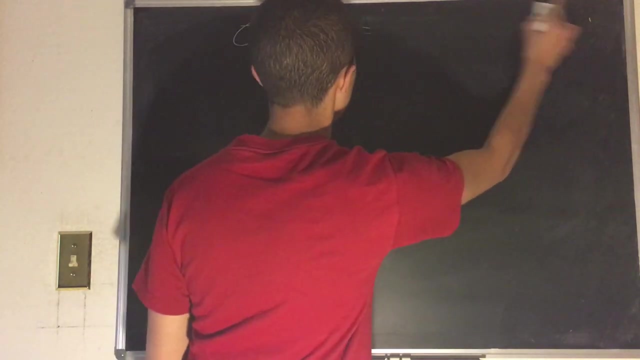 previous cases. So let's prove now That sigma sub k is multiplicative. So let's begin. What we would like to show is that sigma sub k of m n is equal to sigma sub k of m, and times sigma sub k of m And you get the idea. So we will basically start with this. 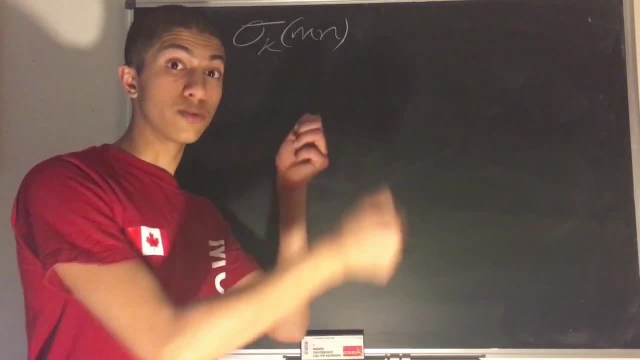 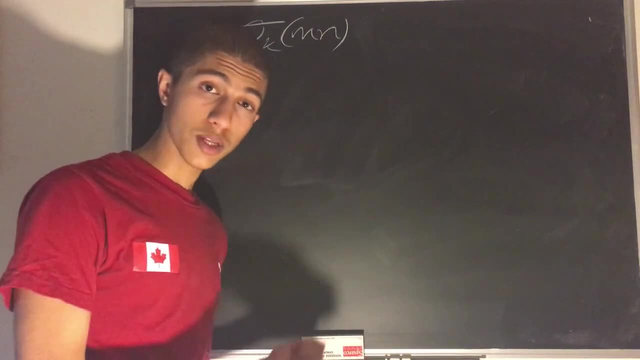 We will start with sigma sub k of m, And we will start with sigma sub k of m And we will start with sigma sub k of m? n, And we will work through steps and simplify or expand And we will come to a point where we have sigma sub k of m times sigma sub k of n, And we'll say, well, this is equal to 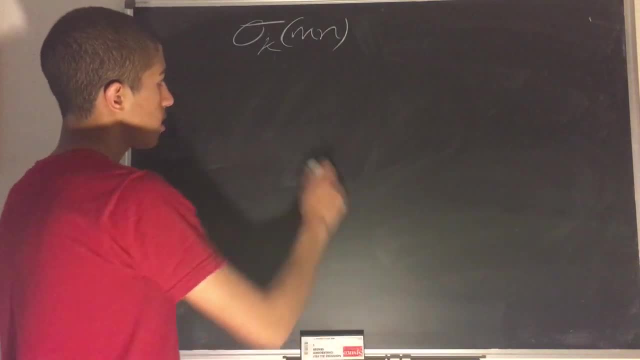 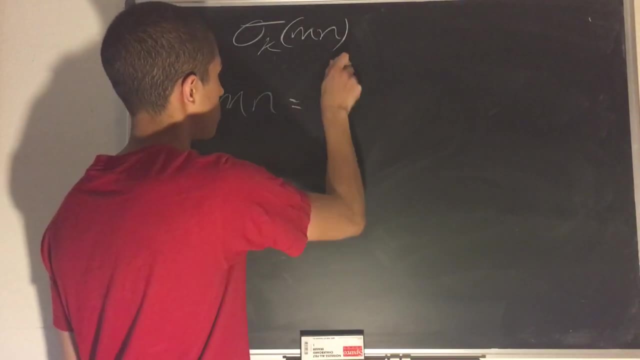 that, And therefore they are multiplicative. So let's begin. Sigma sub k of m n. What does this mean? Well, let's simplify things. Let's say m? n is equal to f And f is just another number, It's. 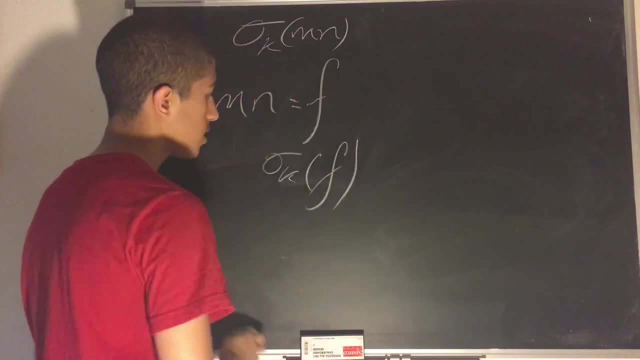 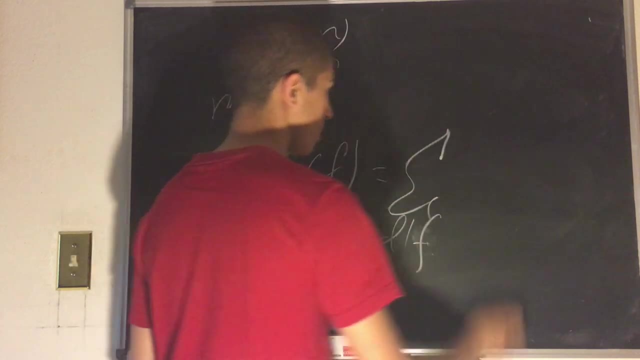 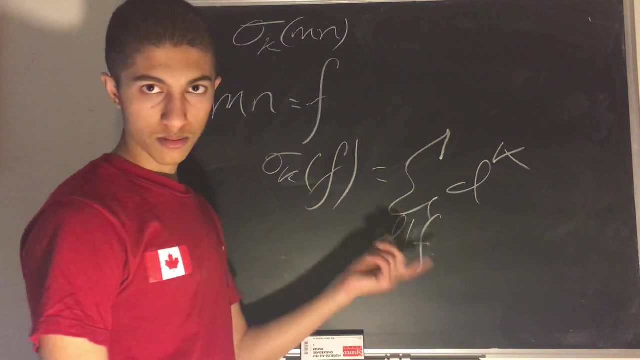 just a number. So let's say: sigma sub k of f is equal to the sum of all d divides f of d to the power of k. Wonderful. So what this is saying is: I'll take all numbers that divide my number f, and I'll 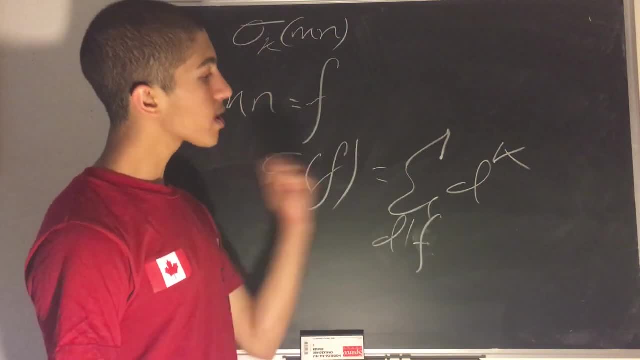 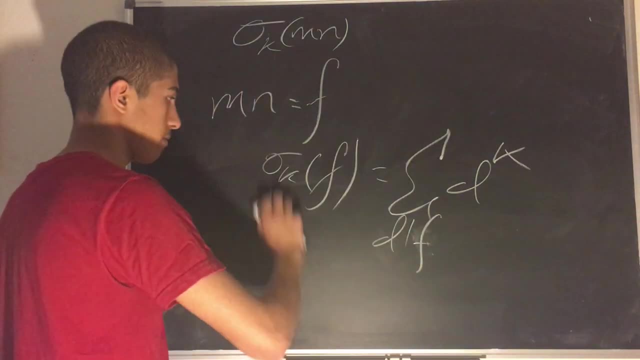 plug them into this sum here And I'll say, okay, I want to take each divisor of f and I want to exponentiate it to some k and add them up And that is what is going to be sigma sub k of f. So 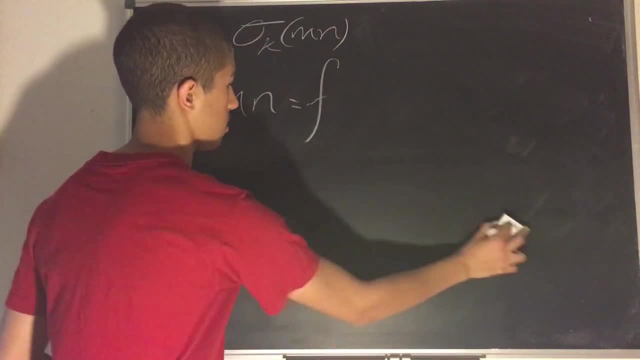 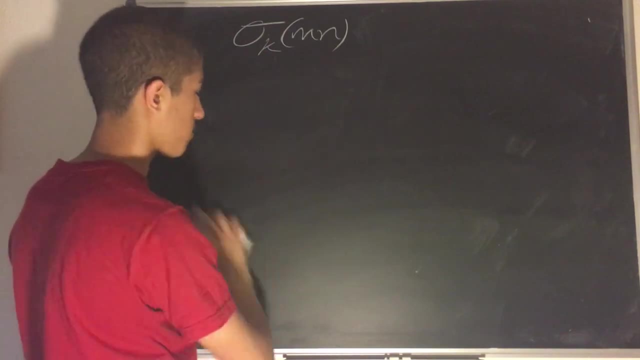 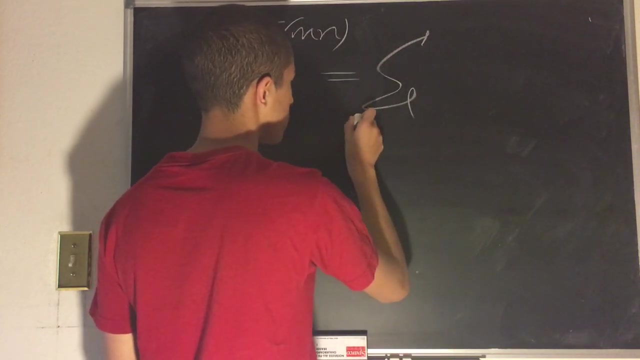 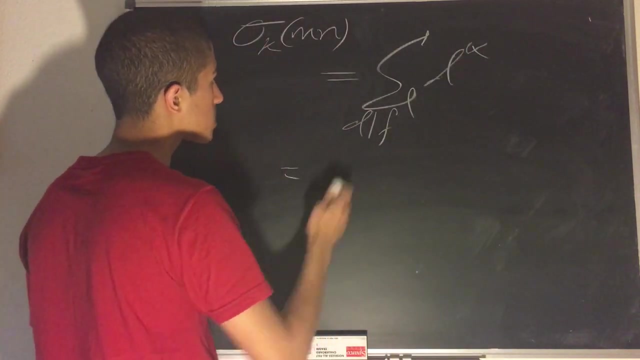 now, what is sigma sub k of m times n? Well, we can break this up. We can say this: sigma sub k of m n is equal to the sum over d divides f of d to the k Right. And well, we can split this up, since 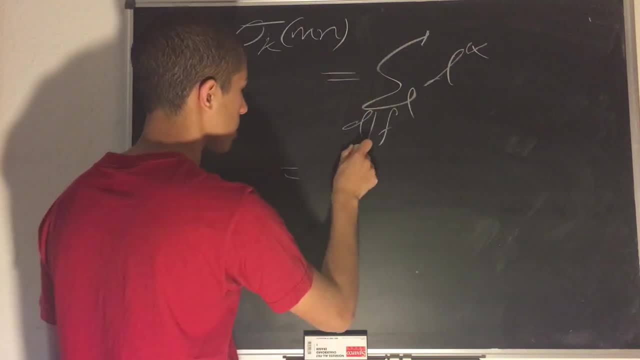 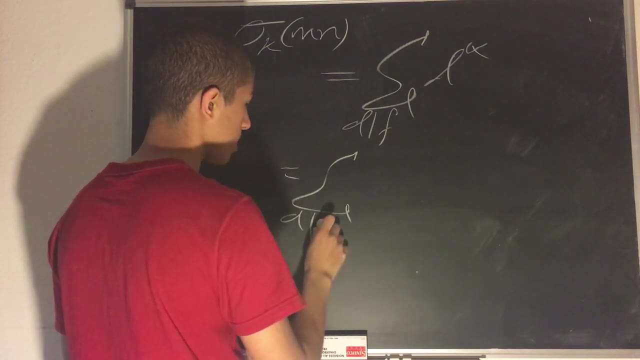 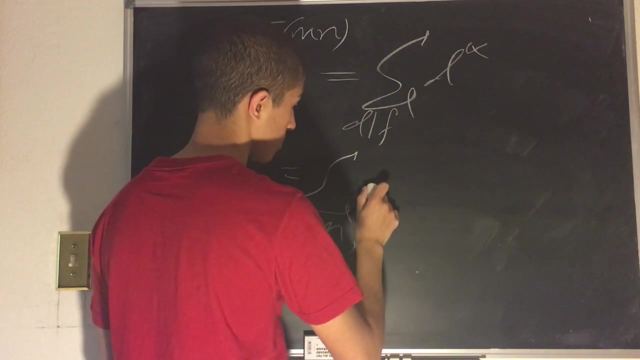 we said: let f equal n times n. We can say, okay, now I'm going to take the sum over both- a divides m and b divides n- of a to the power of k times b to the power of k, And this will essentially equal. 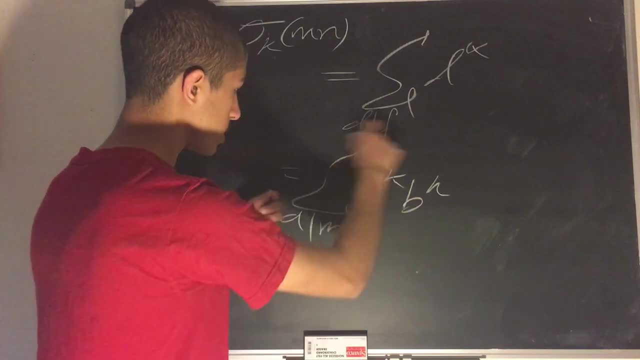 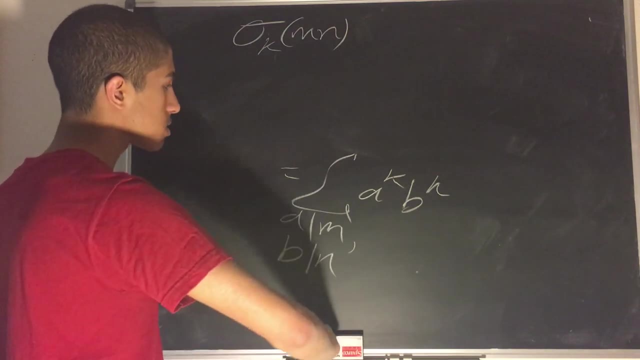 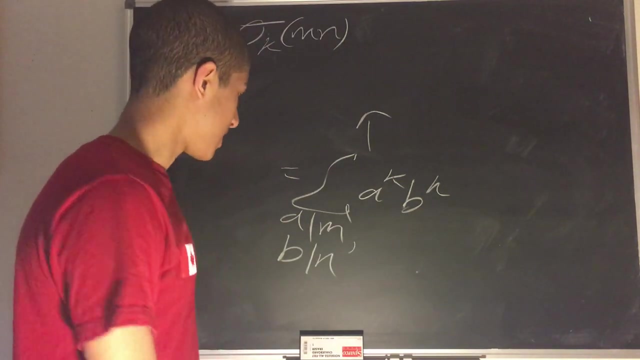 what this is. And well, what is this expression? Well, we can simplify this. Instead of having this weird something comma, something, sigma notation, we can just split it up into a double sum, which is perhaps for you none the more simple, but it is a necessary step in this. 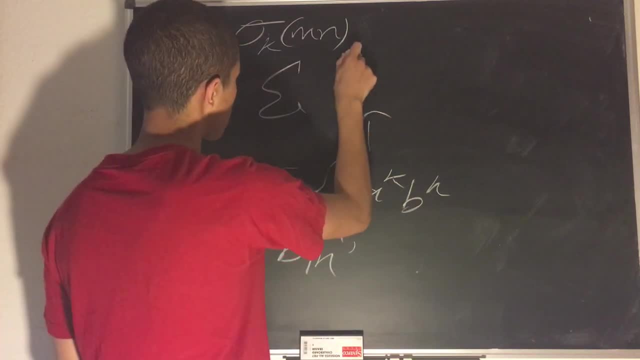 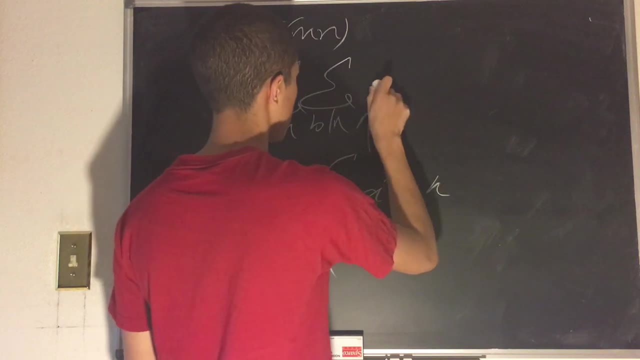 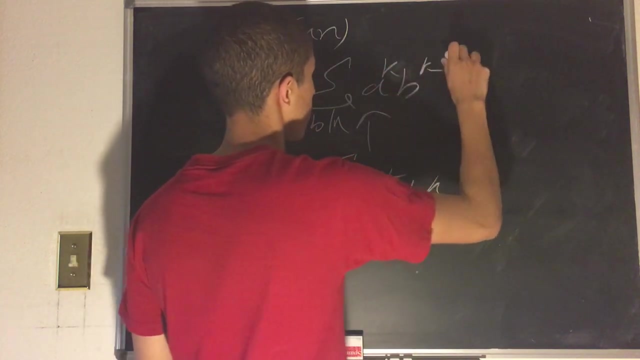 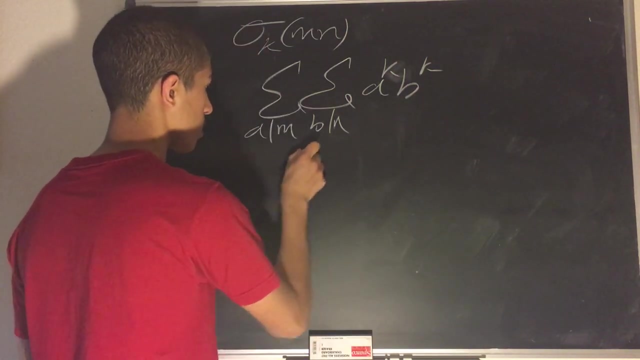 procedure. So we have the double sum over a divides m, b divides n, of a to the k, Or let's say a to the k, b to the k, And then we can simplify this into sigma: a divides m, a to the k. 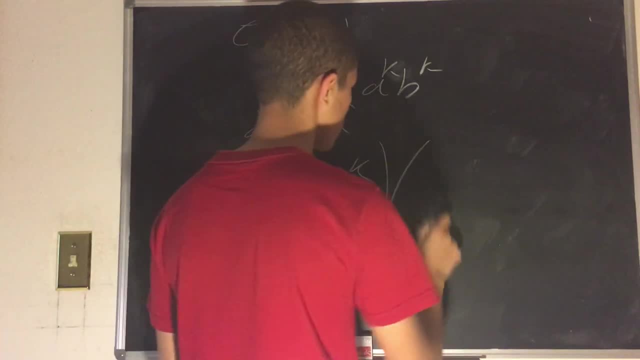 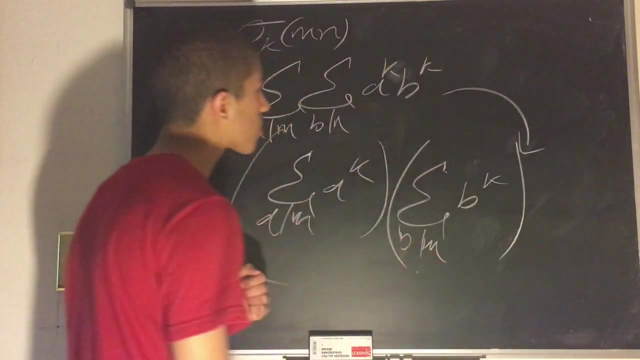 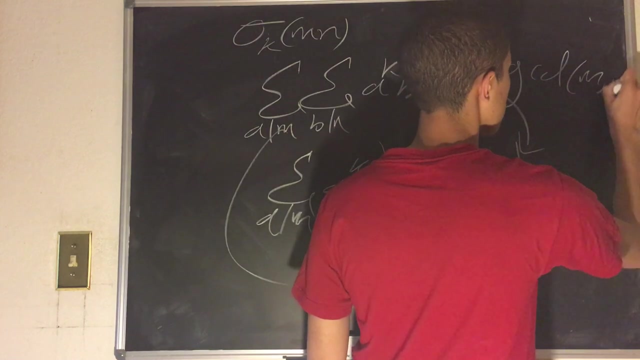 times sigma b divides m, b to the k, And notice that when we make this step, we necessitate that a and b are relatively pro, or that m and b are relatively pro, or that m and b are and n are relatively prime. So here we necessitate that gcd mn is equal to 1.. And now we're basically. 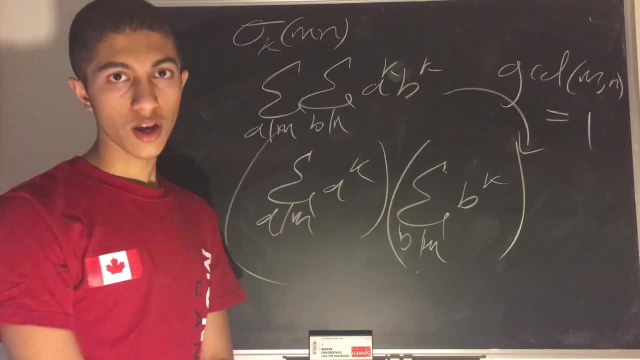 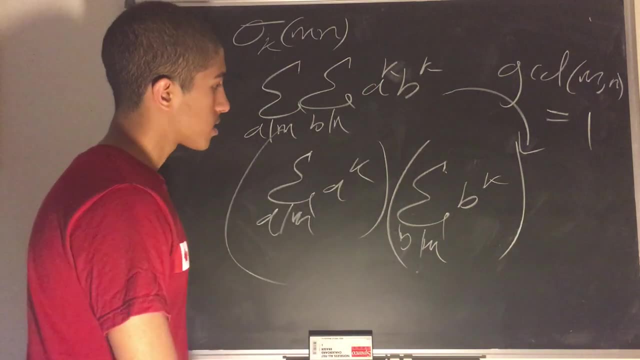 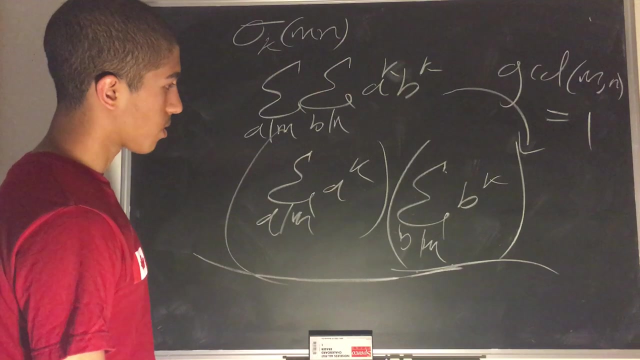 throwing out the notion that this function could be completely multiplicative and we are pushing the notion that it should be simply multiplicative. So then we have this, Oh my god. Then we have this. So what is this equal to? Well, this is very simple, Because, if you recall, 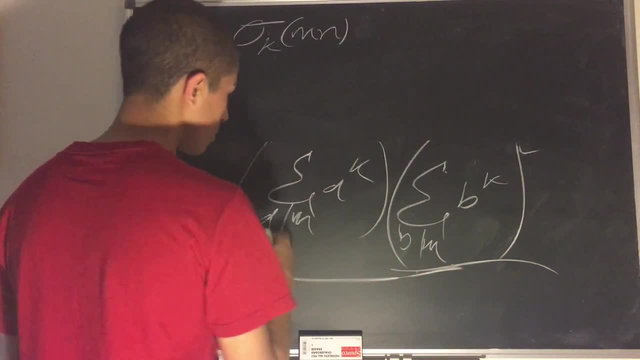 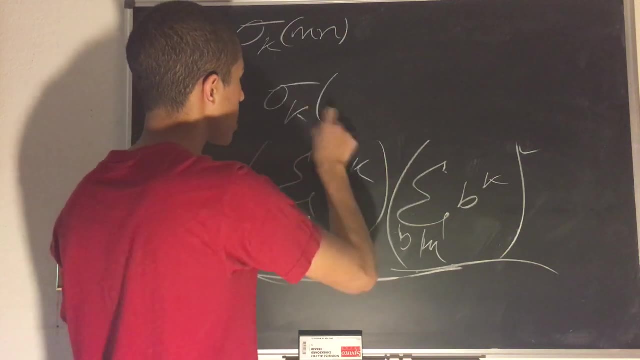 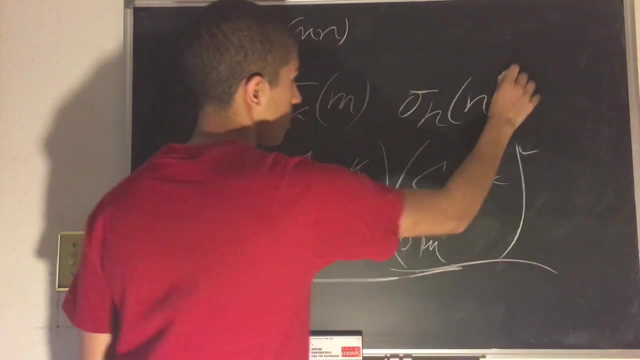 our definition of sigma sub k, it was that you have some d divides, m of d to the k, So this is simply equal to sigma sub k of m times. this is equal to sigma sub k of n. Wonderful, So now we have proved that gcd mn is equal to 1.. And now we're basically throwing out the notion that.